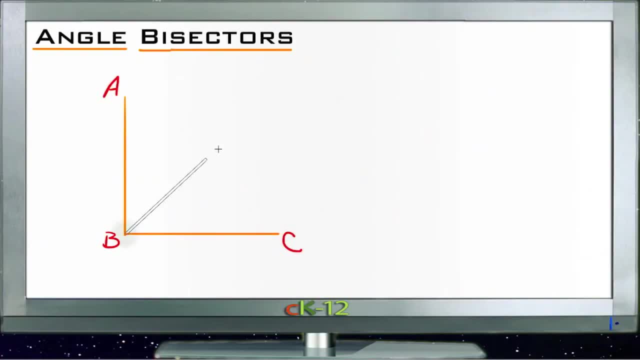 that angle, starting down here at B, off into the ether. here we'll label that ray with a D. here There we go. If the degree measure for ABD is equal to DBC, then this angle, or this line right here, this ray is an angle. 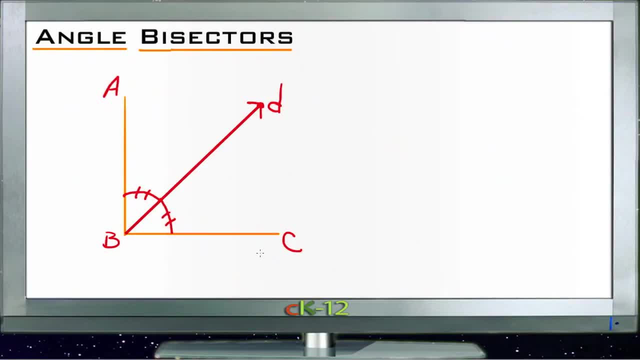 bisector for ABC. It splits angle ABC in half, It bisects it. Now, if that's the case, if you have an angle bisector, then that tells us that any point on the angle bisector line, in this case on D, any time you have a point on that line, if you 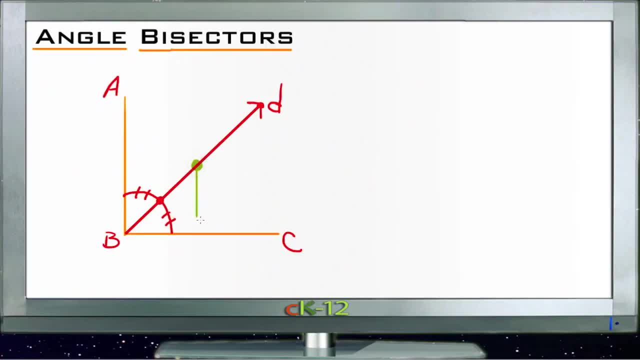 were to draw a line between it and each side meeting each side at a 90 degree angle right here, then each of those two lines is going to be the same. Any point on the angle bisector is the same distance from each of the two other sides of the angle. Now you can use 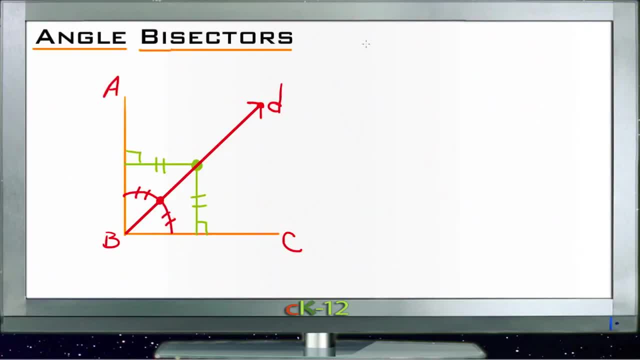 that information in reverse as well. Subtitles by the Amaraorg community. If you, for instance, have an angle and you see that you have a line through it, but you don't know for certain if that line through it actually is an angle bisector, then you: 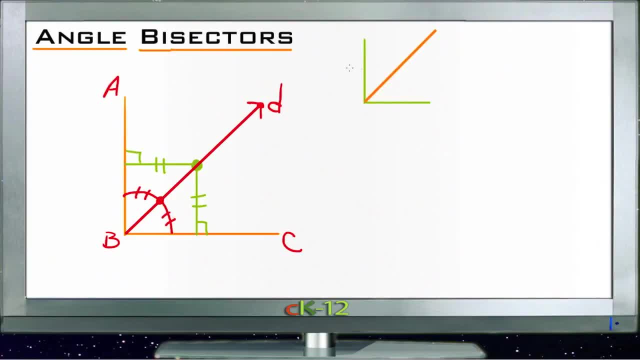 can prove that it's an angle bisector by either showing that the angle measure is the same on either side, like so, or that any point on that line is equidistant from the two sides of the angle. That's called the converse of the angle bisector theorem. Angle bisector theorem tells us that the two distances. 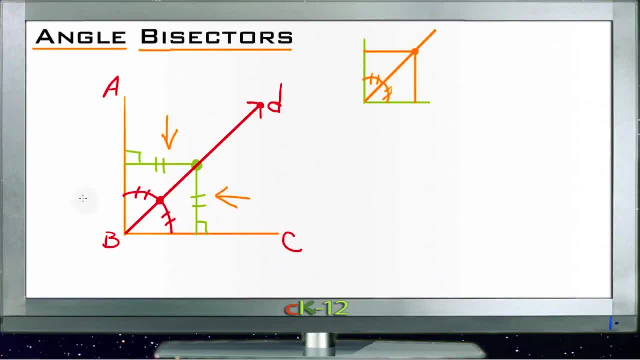 from any point to the sides of the angle are the same and that the degree measures are the same on either side. And then the converse of that theorem tells us that if we can prove that information, then we have an angle bisector. And then, finally, the last thing we're going to talk about here is the application of the 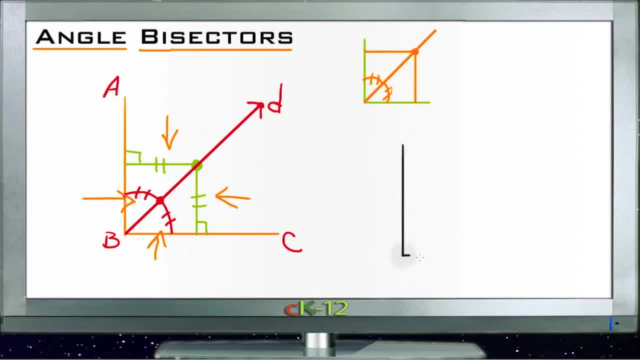 angle bisector theorem to a triangle. If we have a triangle and we have an angle bisector and we apply. let me get my third side there. third side's always a pain because I can't just draw vertical or horizontal lines. if we have a triangle and we go through and